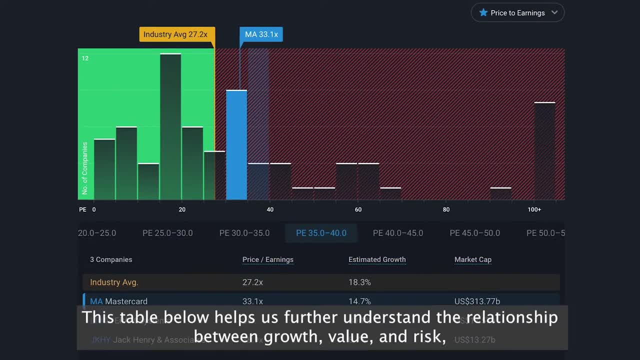 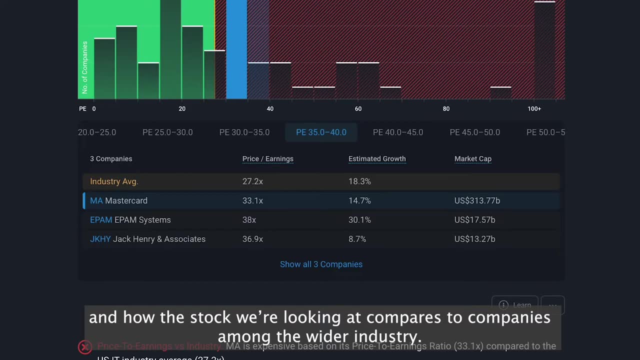 ratio because this company is profitable. This table below helps us further understand the relationship between growth, value and risk and how the stock we're looking at compares to companies among the wider industry. Along the bottom of the chart you'll see the range of. 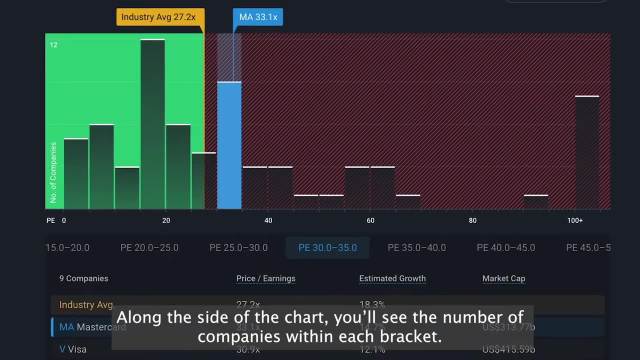 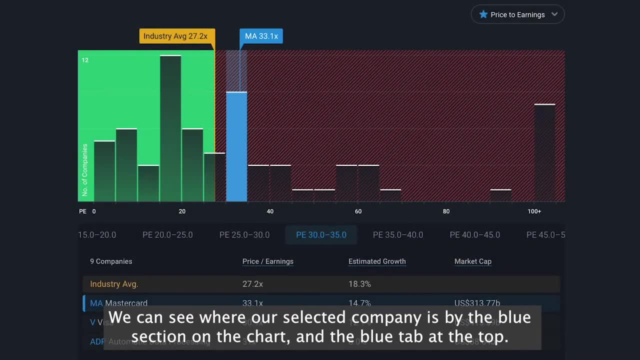 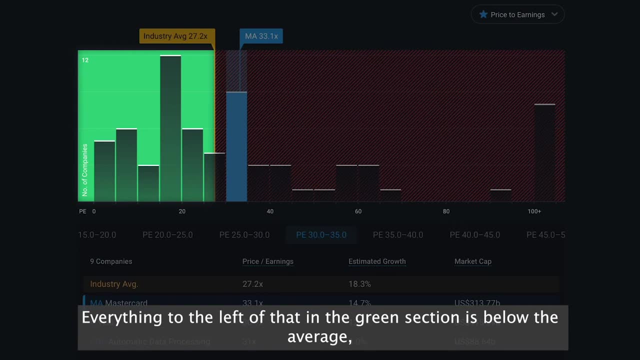 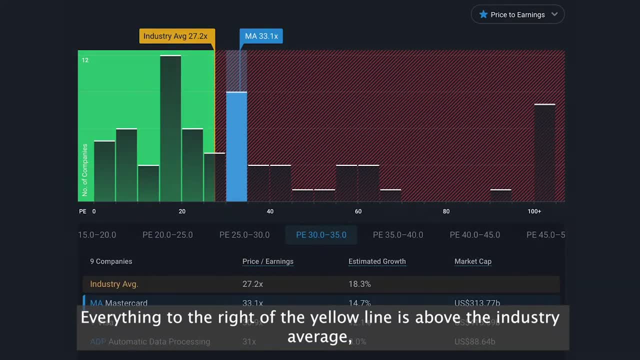 relatively speaking, Everything to the right of that yellow line is above the industry average and indicates that it could be overvalued again on a relative basis. A stock passes this check if its ratio is in the green section, which adds 1pt to its Snowflake valuation score. It fails this. 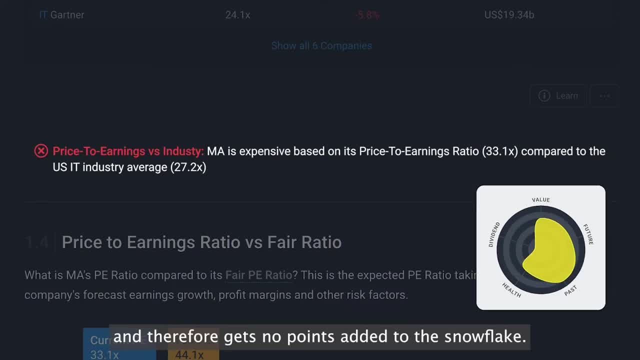 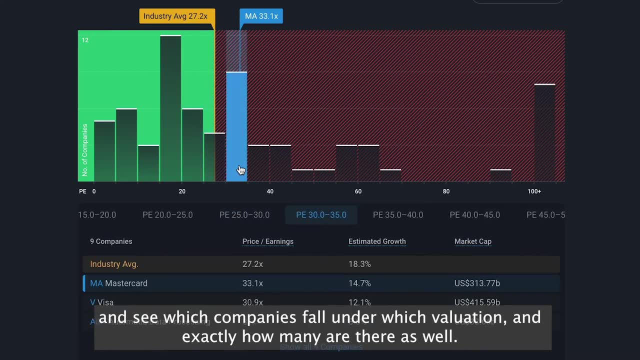 check. if its ratio is in the green section, which adds 1pt to its Snowflake valuation score, It fails. it's in the red section and therefore gets no points added to the snowflake score. to get more detail, we can hover or click each segment and see which companies fall under which valuation. 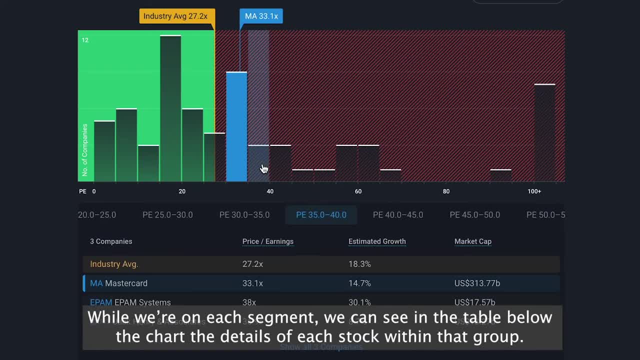 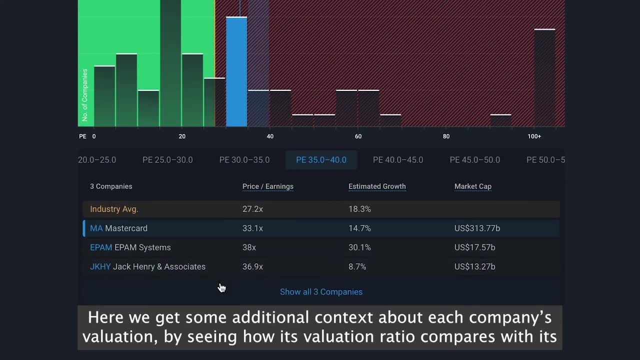 and exactly how many are there as well. while we're on each segment, we can see in the table below the chart the details of each stock within that group. here we get some additional context about each company's valuation by seeing how its valuation ratio compares with its forecasted annual earnings. 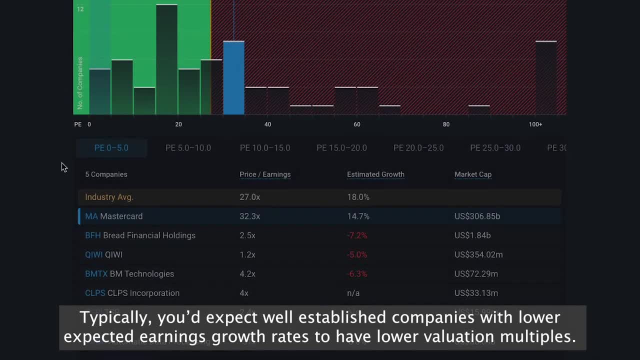 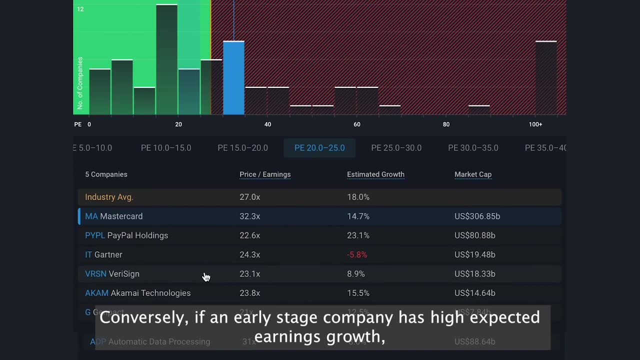 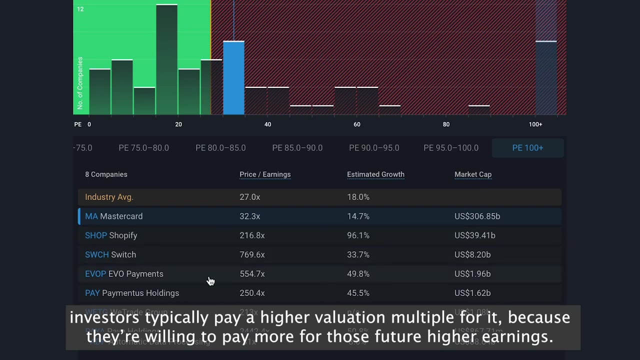 growth rate and its market capitalization. typically, you'd expect to see well-established companies with lower expected earnings growth rates to have lower valuation multiples. conversely, if an early stage company has high expected earnings growth, investors typically pay a higher valuation multiple for it because they're willing to pay more for those future higher earnings.